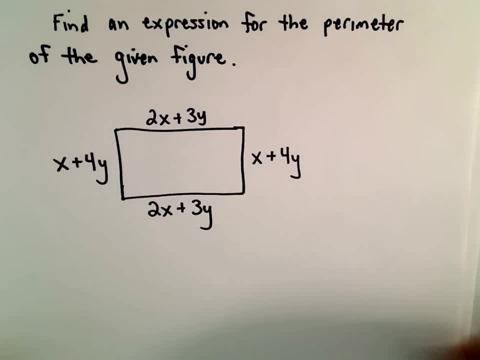 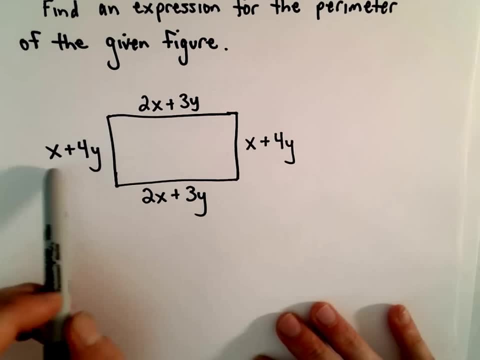 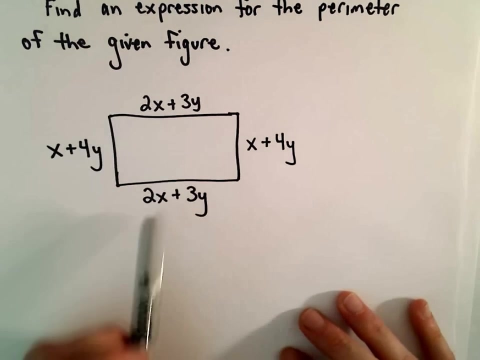 Okay, here we're going to find an expression for the perimeter of our rectangle. So suppose we don't have exact numerical values, but we do have these algebraic expressions. So two of the sides are going to be x plus 4y, x plus 4y, and then the other two sides will be 2x plus 3y and 2x plus 3y. 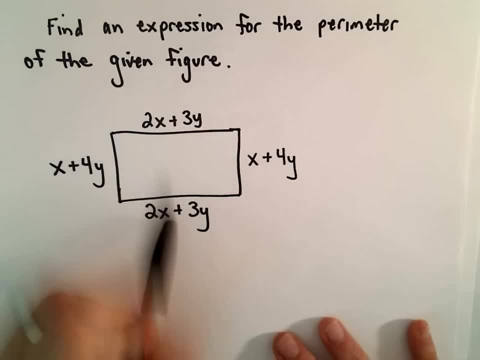 So remember to get the perimeter. we just add up each side. So that's what we're going to have to do in this case: We'll simply have to add up the lengths of these four sides and of course, we'll try to simplify this expression down. 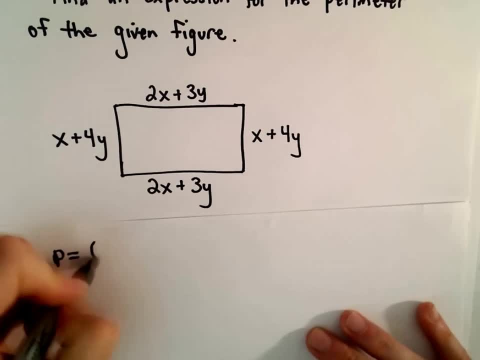 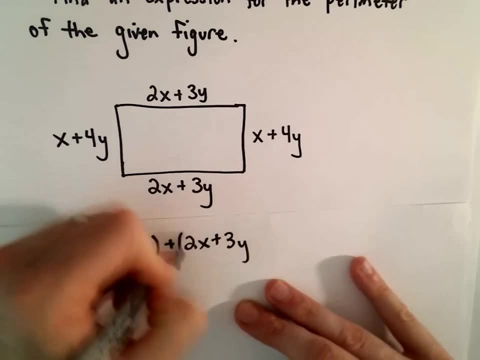 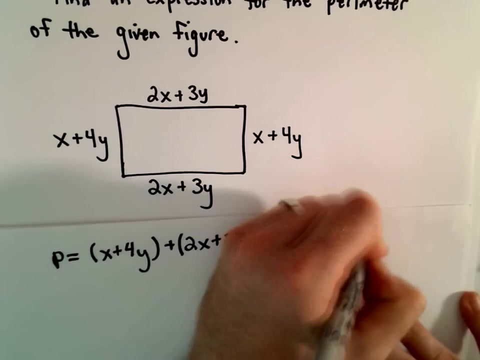 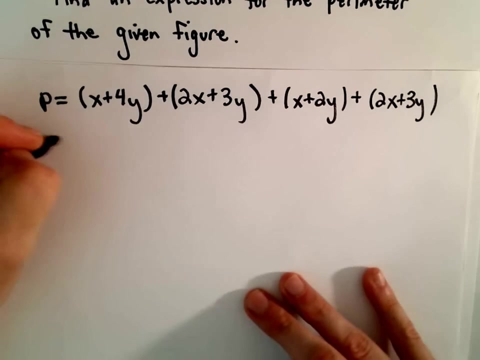 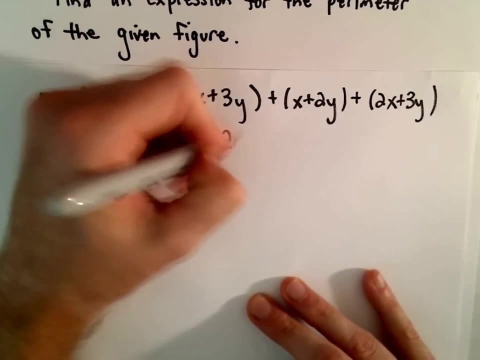 So the perimeter P, that'll be x plus 4y plus 2x plus 3y plus x plus 4y. Again, you could have also said this a little differently. We could say: we have two times the side x plus 4y. Likewise we have two of the sides, 2x plus 3y. 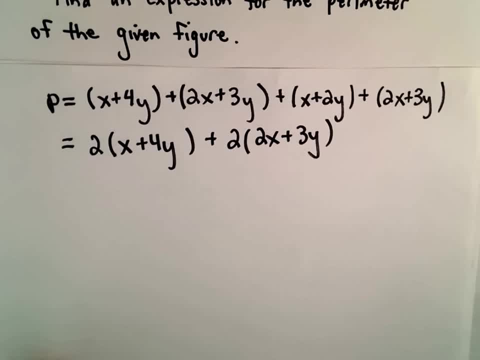 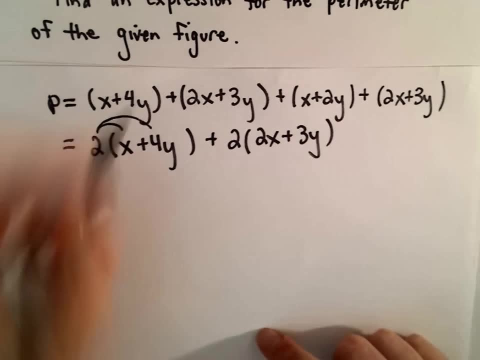 So either one of those expressions are absolutely correct. Probably the second one here is even a little bit easier to see. Well, maybe not. I guess it's all the same difference really, But I'm going to go ahead and do the work on this expression. 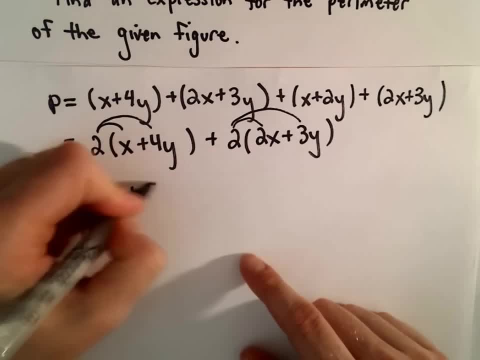 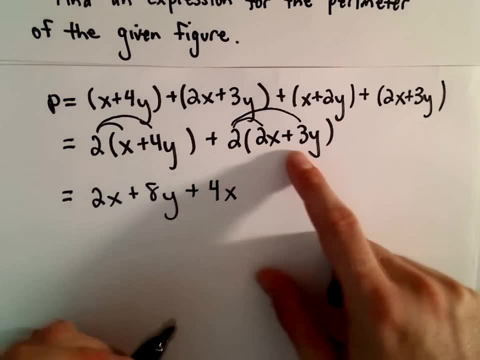 So we have 2 times x, 2 times 4y, which will be 8y, 2 times 2x, which will be 4x, 2 times 3y, which will be 6y, and now it's just a matter of combining like terms. 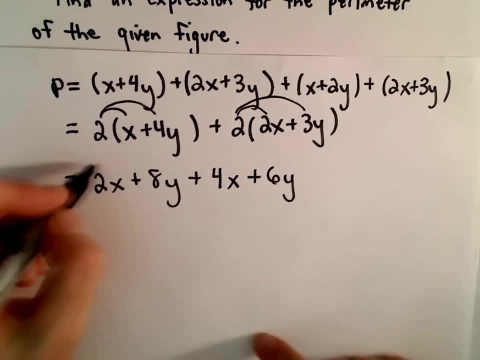 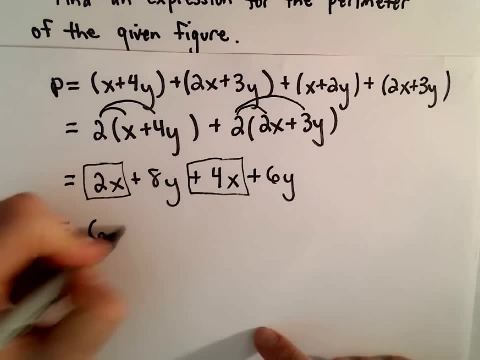 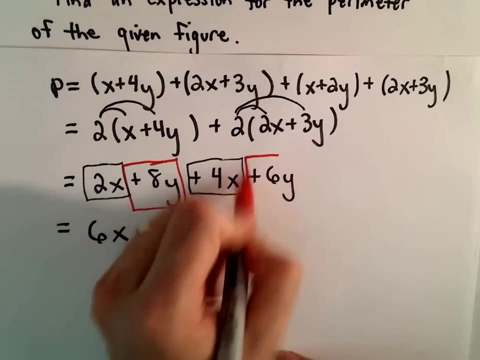 I see something involving x to the first power and x to the first power. So we can combine. So we can combine those two terms. 2 plus 4 will give us 6.. Again, we keep the x And then again we have some more like terms. We have a positive 8y and a positive 6y. 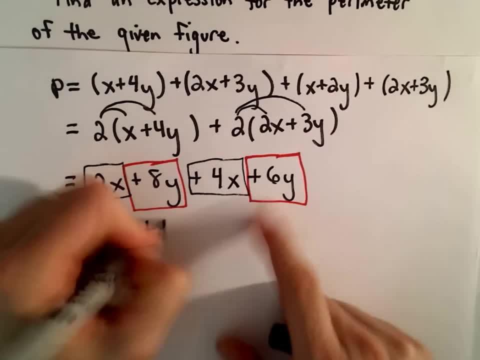 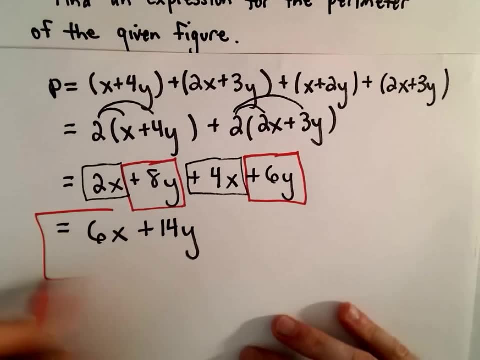 Well, positive 8y plus 6y will give us a positive 14y. And again at this point, x and y are not like terms, so we can't combine those any further, and that would be our simplified expression.